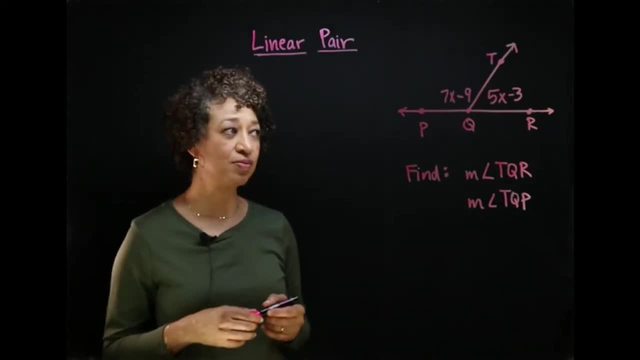 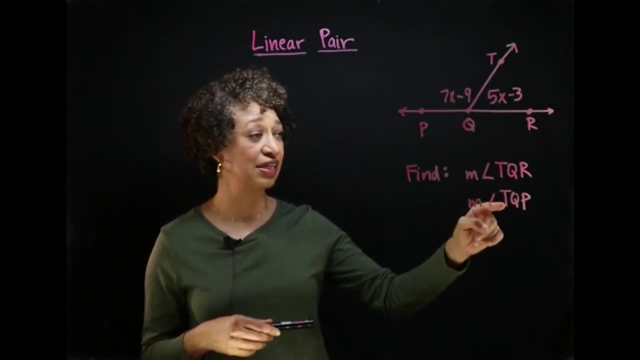 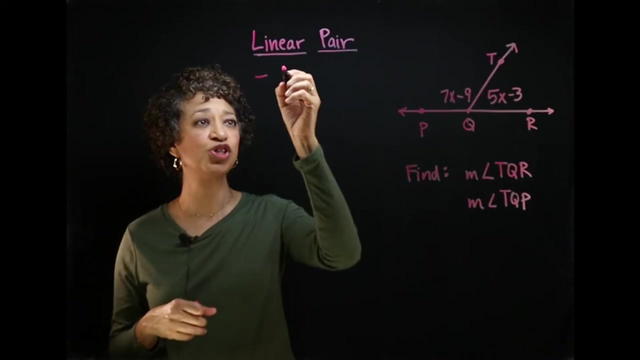 what to do in each of these situations. So my first problem is with a linear pair. We are asked to find the measure of angle TQR and the measure of angle TQP, But I want to review first what a linear pair is. A linear pair is, first of all, two adjacent angles. 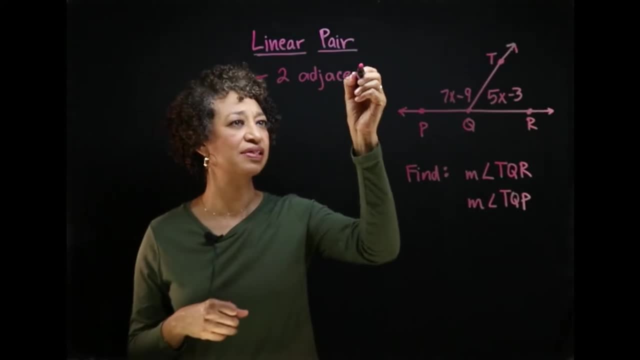 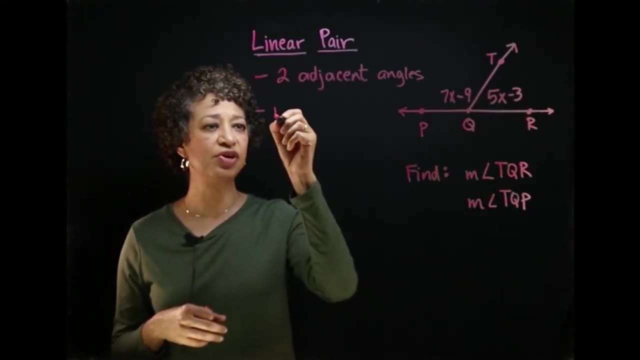 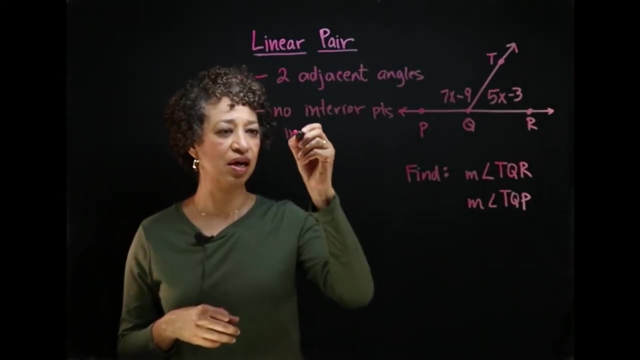 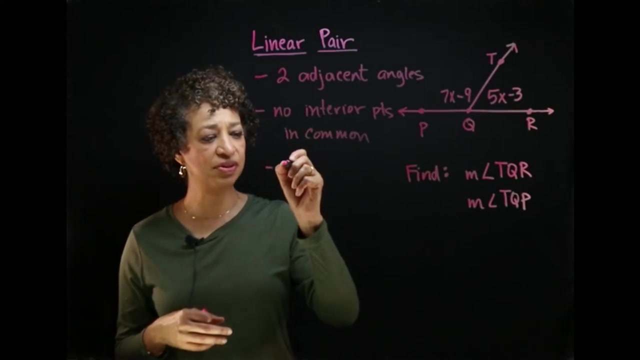 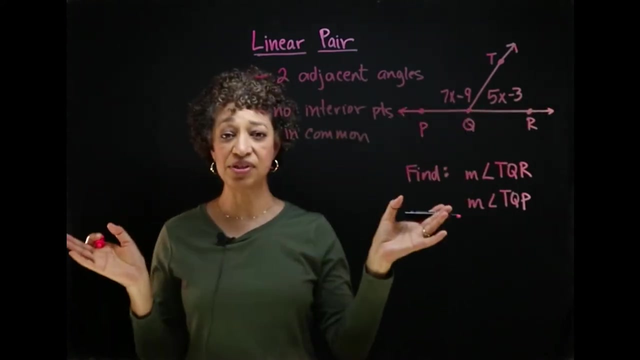 Two adjacent angles. Adjacent just means side by side. It means that they're side by side. They have no interior points in common. No interior points in common. And thirdly, they have opposite rays that make a straight line. This ray, ray QR and ray QP are opposite rays. They 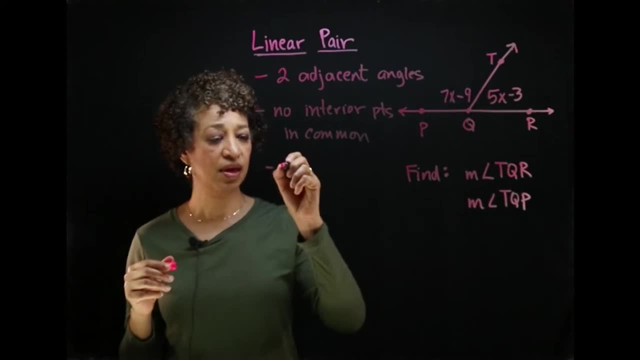 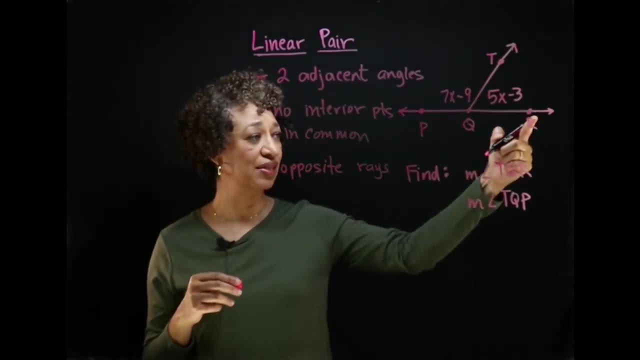 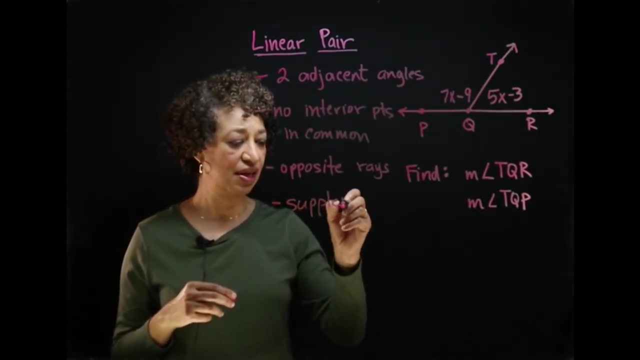 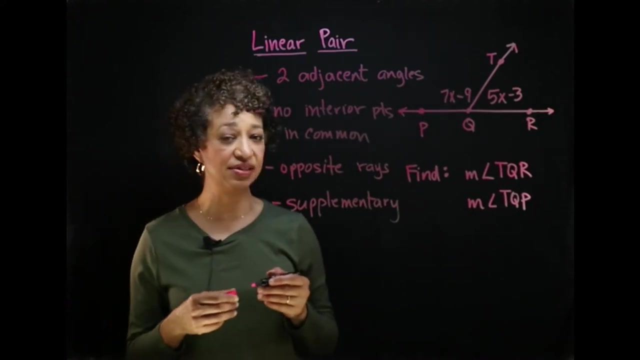 make a straight line, So they have opposite rays And since those are opposite rays, we can say that these two angles add up to 180 degrees. They are supplementary. The angles in any linear pair will be supplementary. They will add up to 180 degrees. So, with this in mind, let's solve this problem Now, since our pair 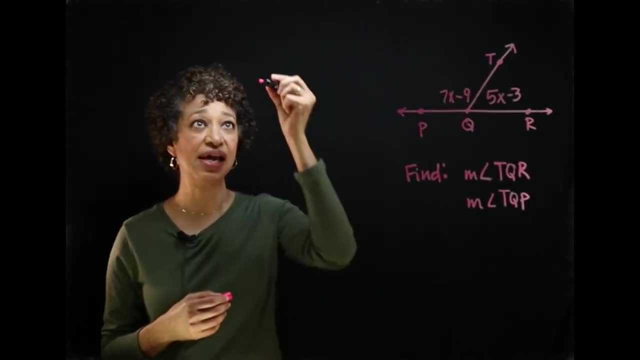 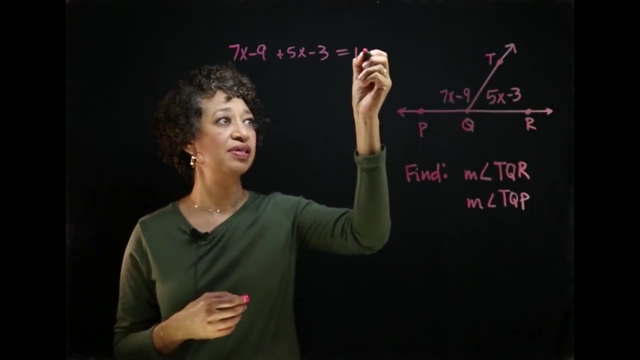 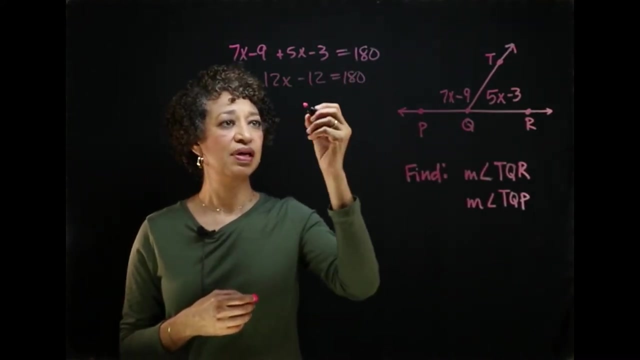 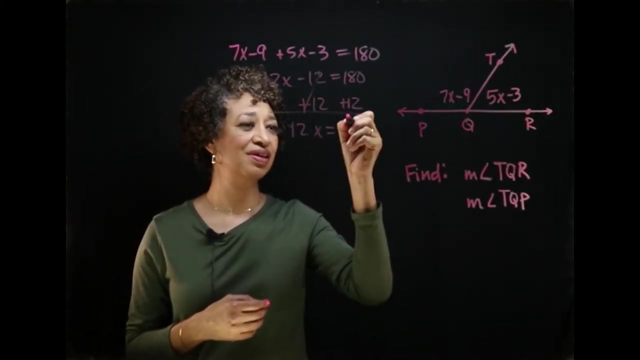 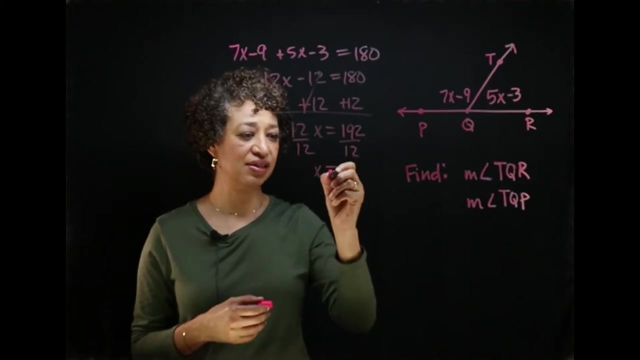 of angles is supplementary. we know they will add up to 180 degrees. I'm going to add them together and set them equal to 180 degrees. I'll combine like terms. I will add 12 to both sides And I have 12. X is equal to 192.. Now, dividing both sides by 12, I have X is. 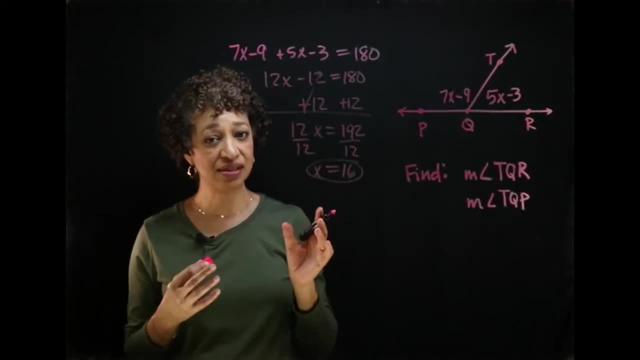 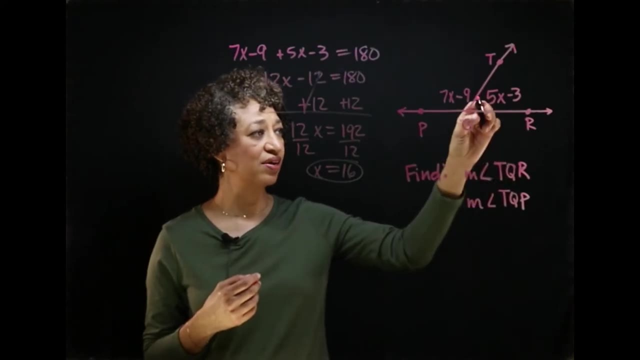 equal to 16.. But that is not what they asked for, So I'm going to add up to 120 degrees. ask us to find. We need to find the measure of angle TQR. That's here, So I'm going to. 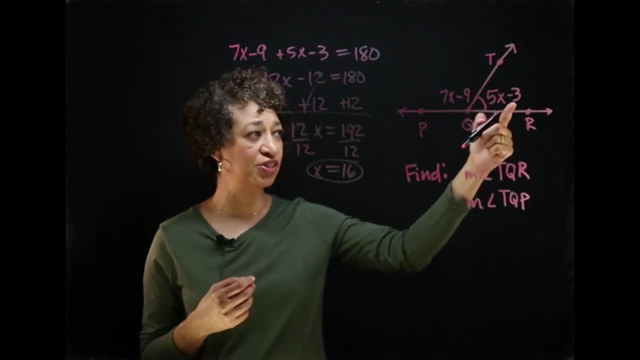 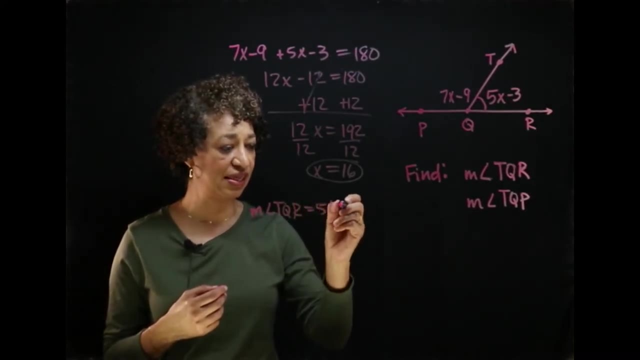 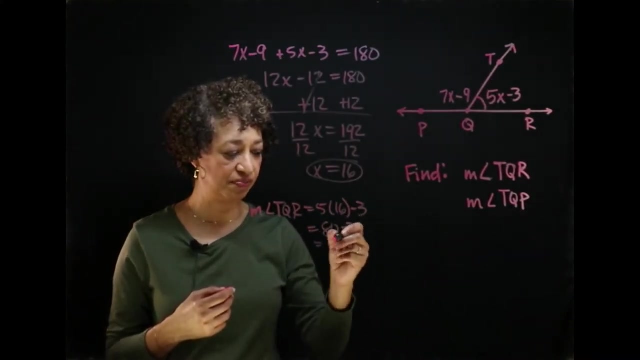 plug in my 16, where I see an X in this expression. So then the measure of angle TQR is equal to 5 times 16 minus 3,, which is 80 minus 3,, which is 77 degrees. Okay, Now I need to get. 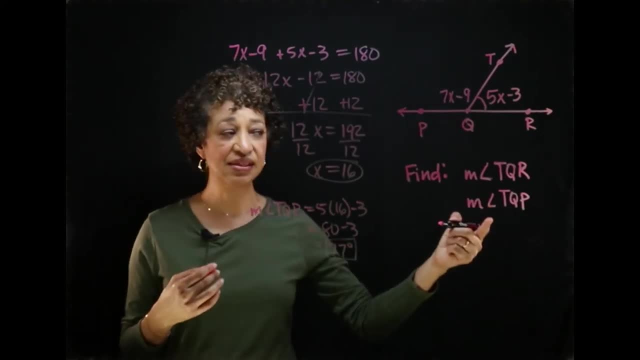 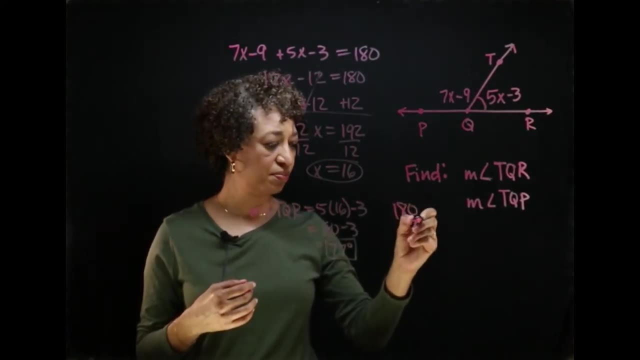 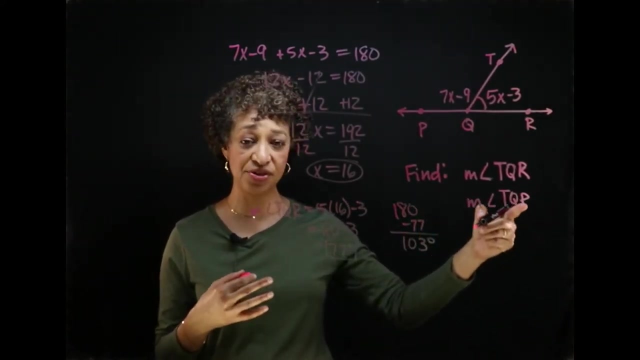 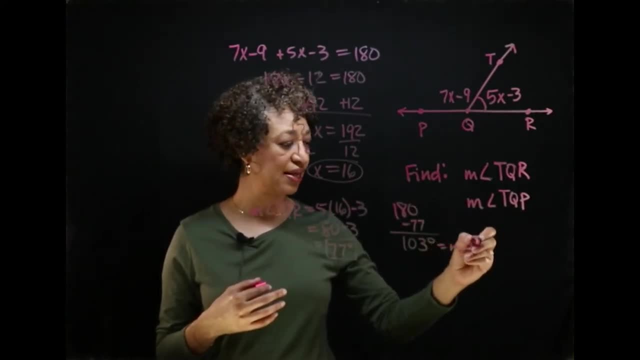 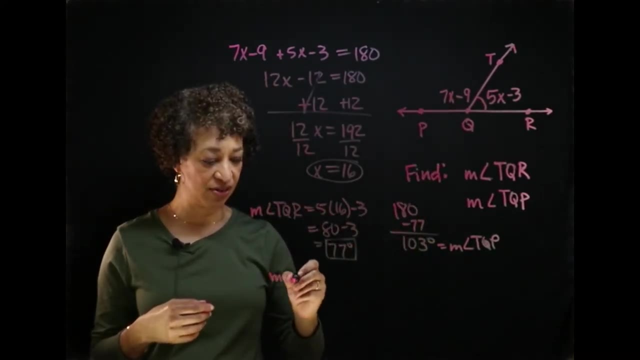 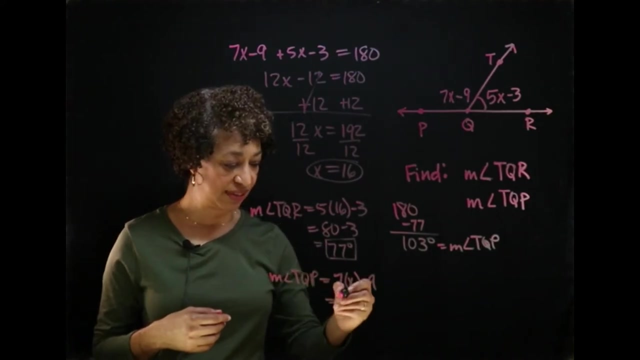 103.. But let's just plug it in to the expression for TQP to verify. Okay, So the measure of angle TQP is 7X minus 9,, which is 7 times 16 minus 9,, which is 112 minus 9,, which is: 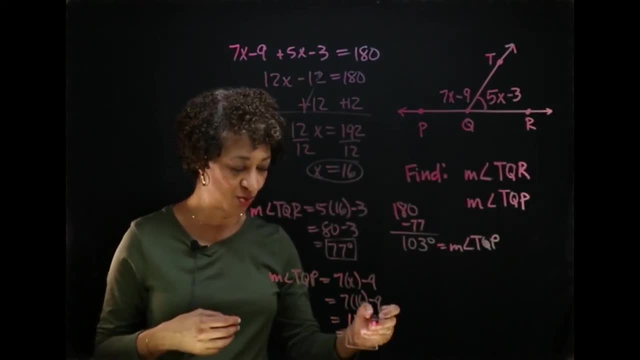 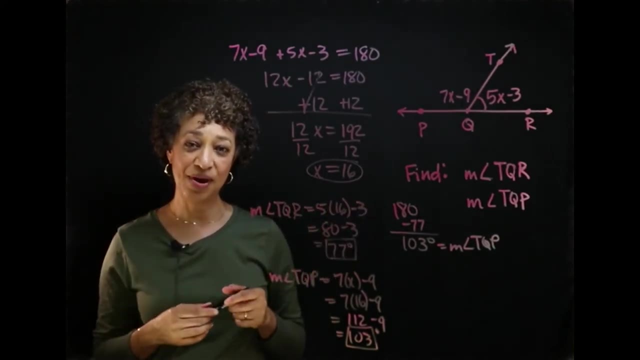 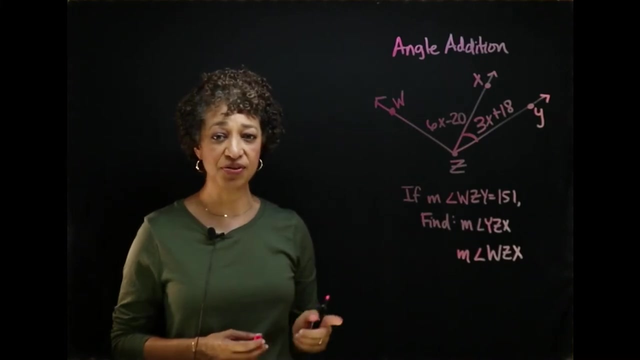 103.. Yay, That is correct. That is what we expected and that's what we got. So this is the problem involving a linear pair. Now our second problem involves angle addition. It is very much like the first one we did, except the first one was a linear pair and therefore those angles were supplementary. 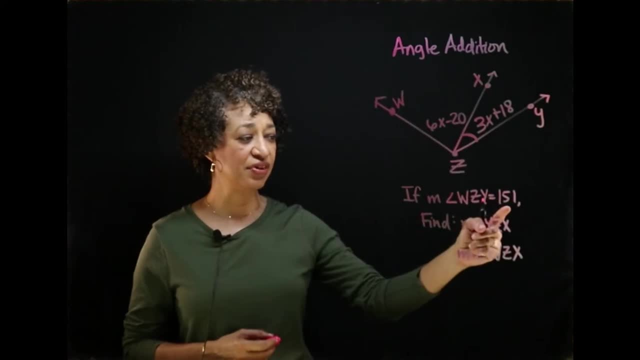 This time we will still add the angles together, but we are given 151 as the total measure of the two angles. Okay, So we're going to add the angles together. We're going to add the angles together. So we're going to add the angles together. We're going to add the. 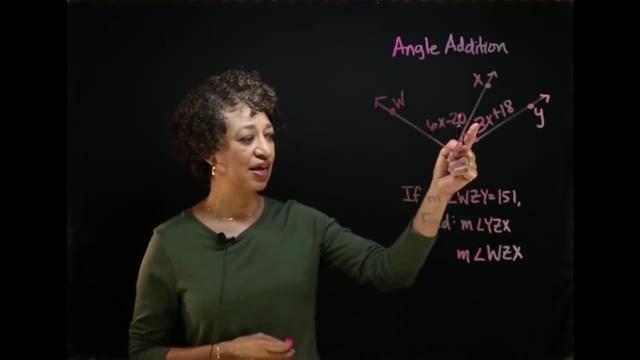 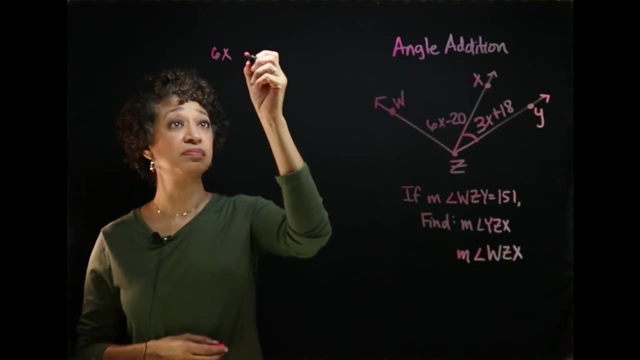 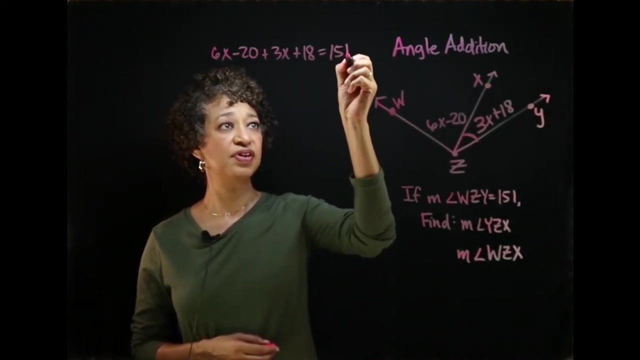 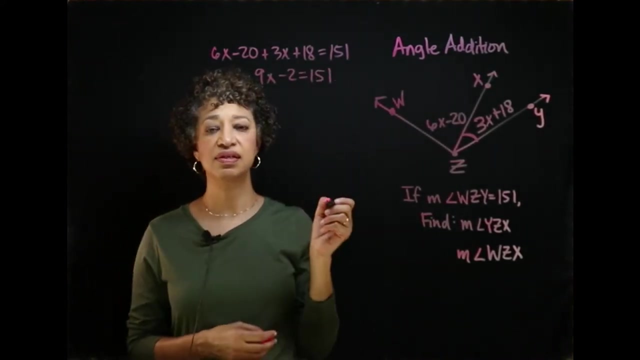 angles together. Okay, So we're going to add the two expressions and set them equal to 151 this time. So I have 6X minus 20 plus 3X plus 18 is equal to 151.. Again, combining like terms, we have this: Adding 2 to both sides, we end up with: 9X is equal to 151.. 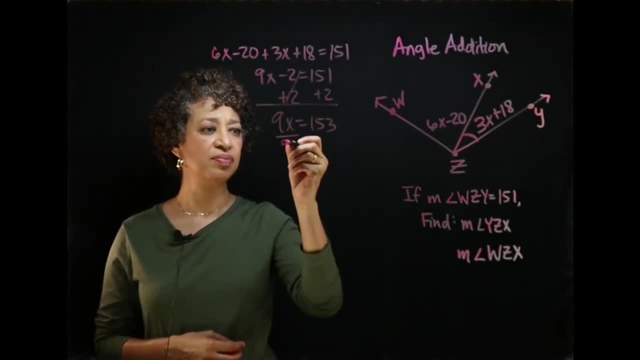 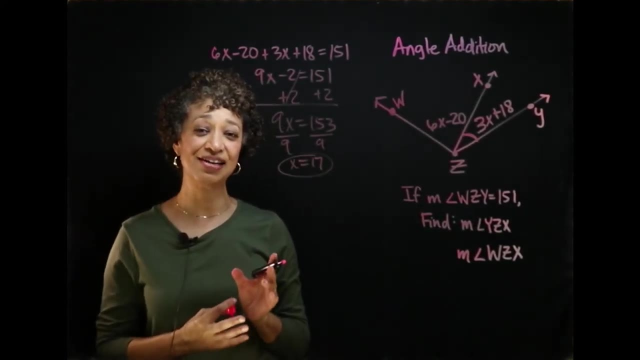 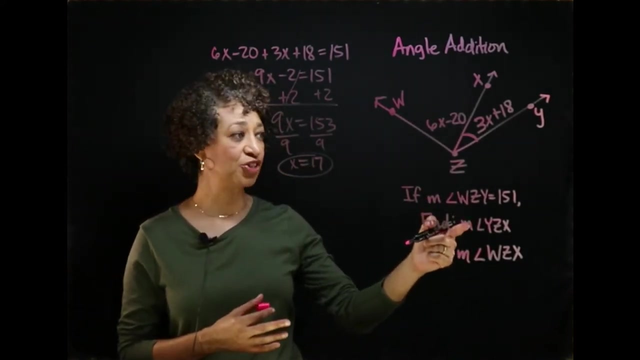 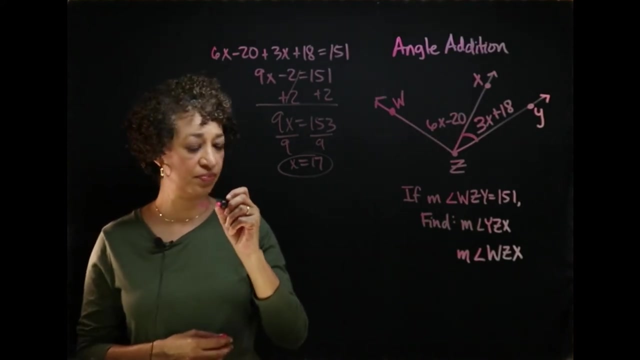 X is equal to 153, and dividing both sides by 9, we get X is 17.. But again, we were not asked to find X. We will just need to use X in order to get the measure of these two angles. First, the measure of angle YZX: It's 3X minus 18.. So I'm going to plug in. X equals 17 into 3X minus 18.. Okay, So I'm going to plug in X equals 17 into 3X minus 18.. Okay, So I'm going to plug in X equals 17 into 3X minus 18.. Okay, So I'm going to. 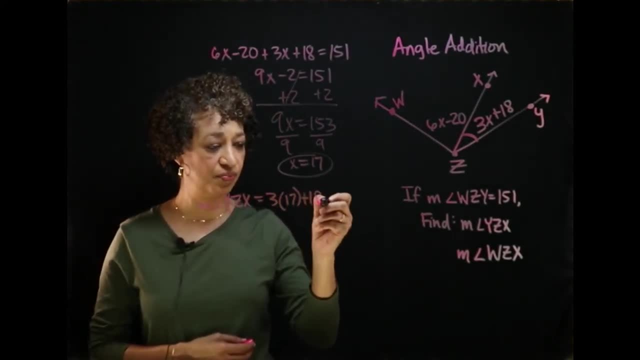 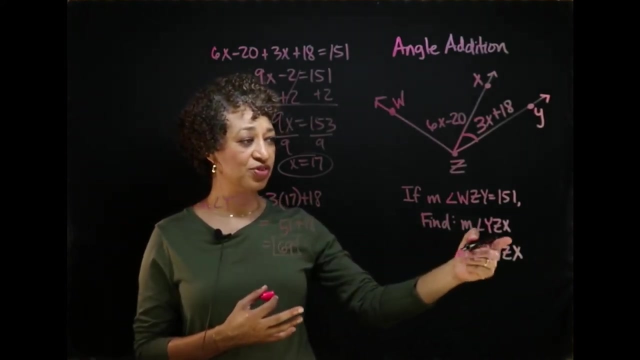 plug in X equals 17 into 3X plus 18.. We get 51 plus 18,, which is 69.. That is the measure of angle YZX. Now, in order to get the measure of angle WZX, since the total is 151,, we really. 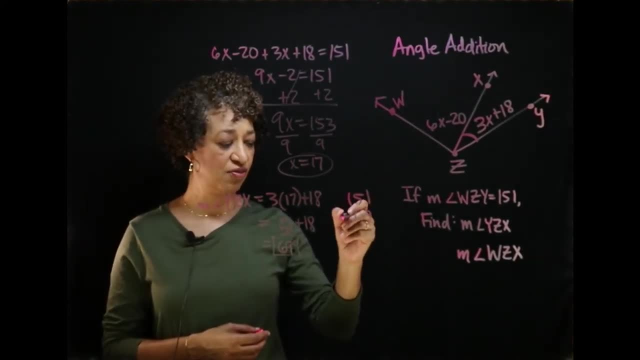 could just subtract 69 from 151 and get 82.. 82 is the measure of angle WZX. So we're going to plug in: X equals 17 into 3X plus 18.. Okay, So I'm going to plug in: X equals 17 into 3X. minus 18.. Okay, So I'm going to plug in 17 into 3X plus 18.. Okay, So I'm going to plug in X equal 17 into 3X. Okay, So I'm going to plug in 17 into 3X plus 18.. And that gives. 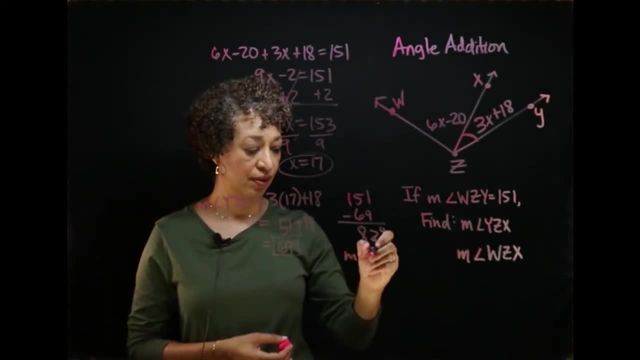 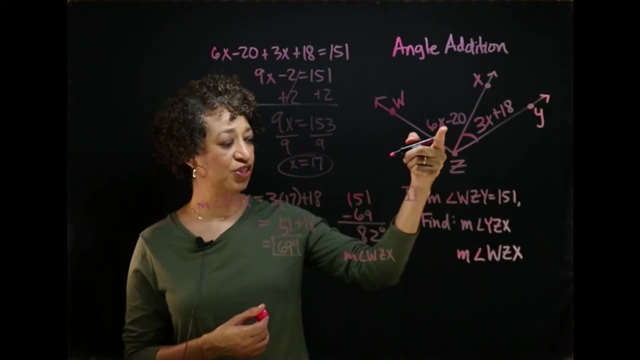 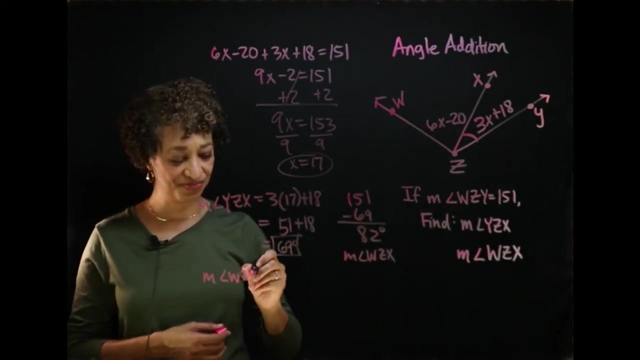 Los Angeles. So stiff, Okay. So I'm going to plug in, we'll get 32 because, אומר remlin wilden him, we went with 32 for those angles, Okay. So essentially the formula for little m capable is WZX plus 19.. And I will just plug in 17 to resolve for that. 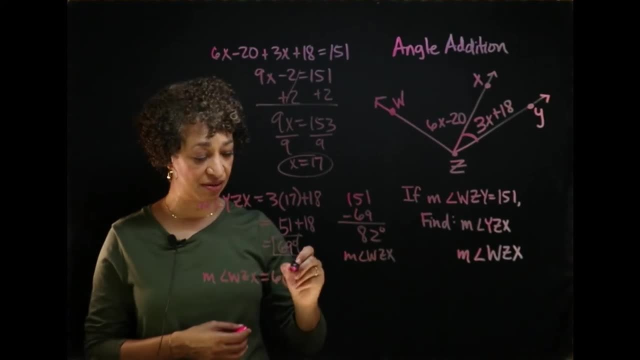 question. Okay, So inside thisificar here, as far as the dollars are concerned, I'll also plug in 17 to resolve for what I get, And it does include what I've added into this, which was March 26th: Galaxy L versus 14.. Now here's one of the 71 cents I'm going. 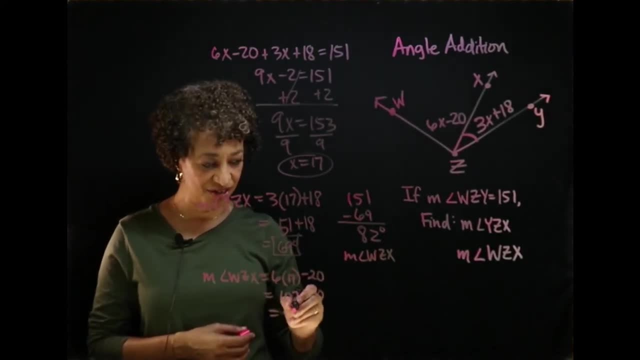 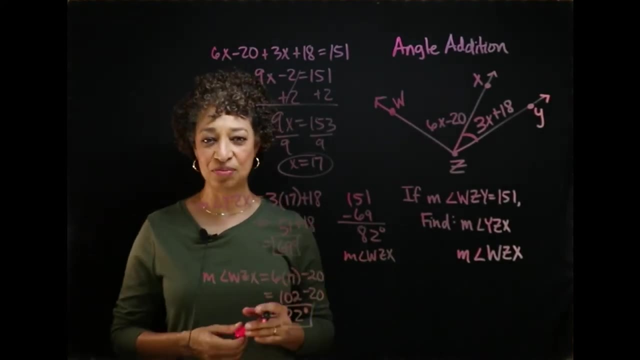 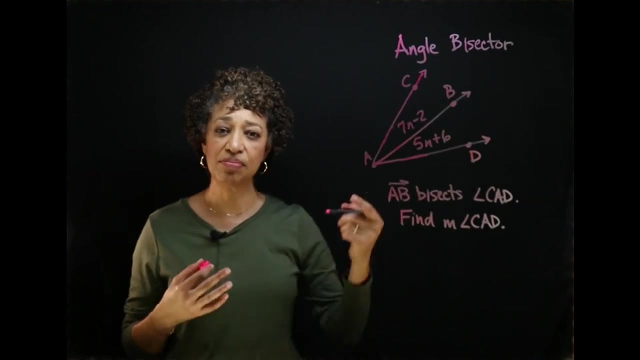 to find 20 for first, and what happens if I do find 12 in here? My answer is H, which is 82, and you see that we get the same thing. Yay, Okay, so that is the second problem. Now our third problem involves an angle bisector To bisect, of course. 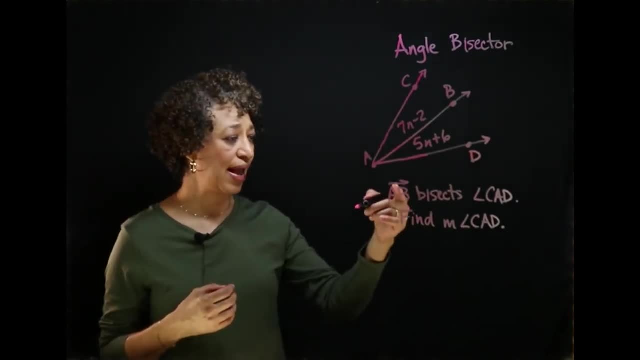 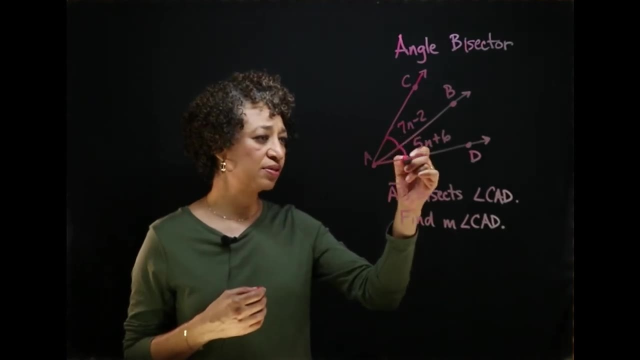 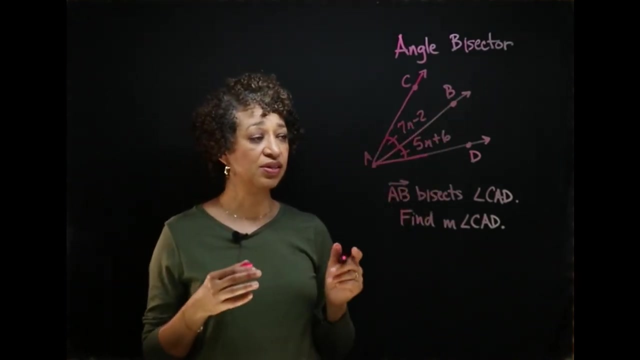 means to cut in half. We are told here that ray AB bisects the larger angle, CAD, So I know that these two smaller angles will be congruent. They will have the same measure because the ray bisects the larger angle. So instead of adding these, 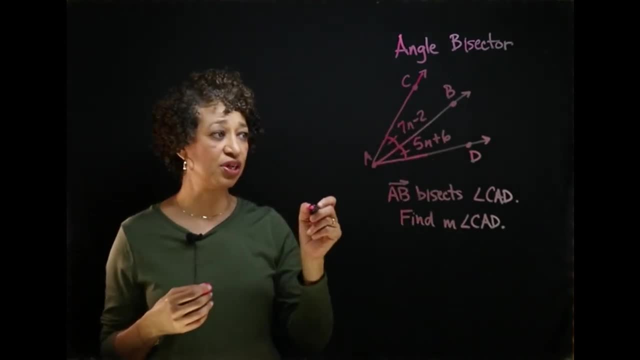 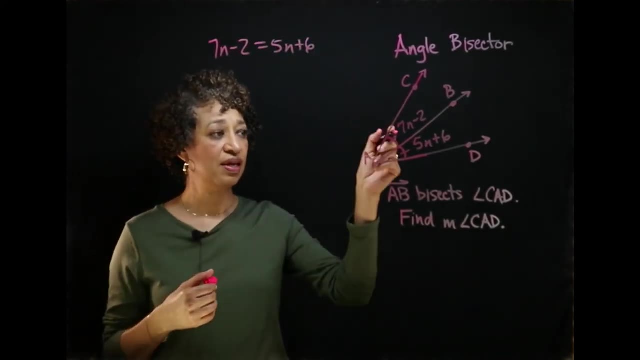 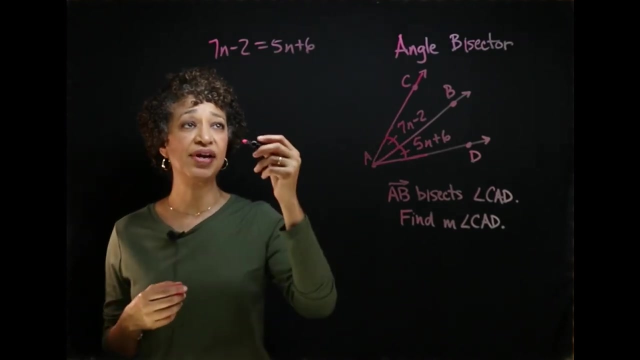 two expressions together. I'm going to set them equal to each other. We have: 7n minus 2 is equal to 5n plus 6.. The angles will have to be equal again because AB is a bisector. Alright, I'm solving for n. I'm going to subtract 5n from both.